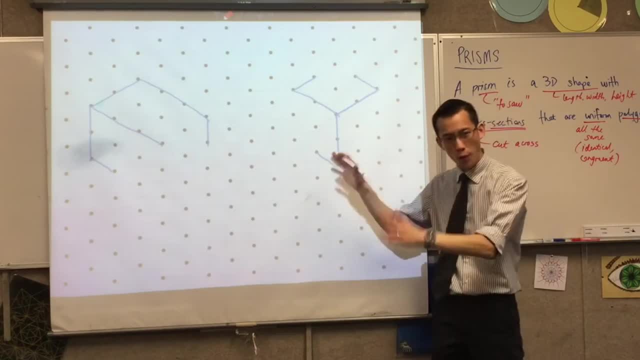 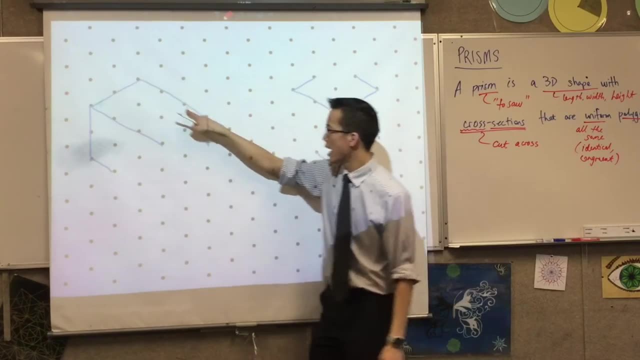 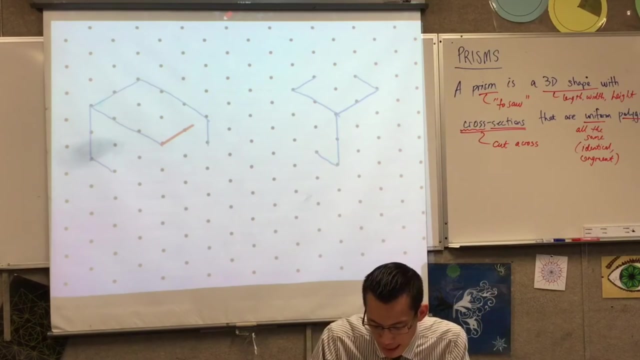 Secondly, the cross sections ought to be uniform. So, for instance, can you see how, across this way, the edge it ends, This edge ends and then it starts going down? Well, if that's the case, in order to keep it uniform, I have to have a corresponding edge over here. You see that, Otherwise I'm not going to get uniform cross sections. 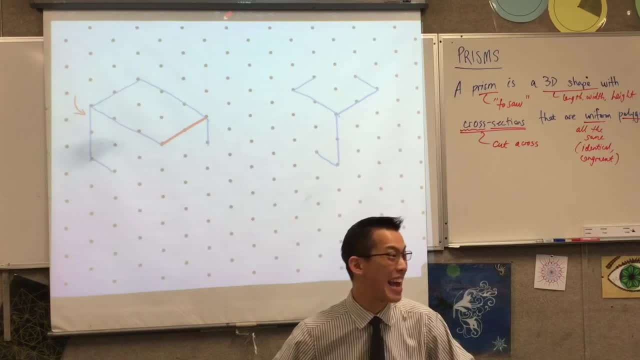 In the same way. you see how this edge that's right here on the left-hand side, you see how it goes down two units. So that means all of these other edges must also go down two units with it, And then you can pretty much see. 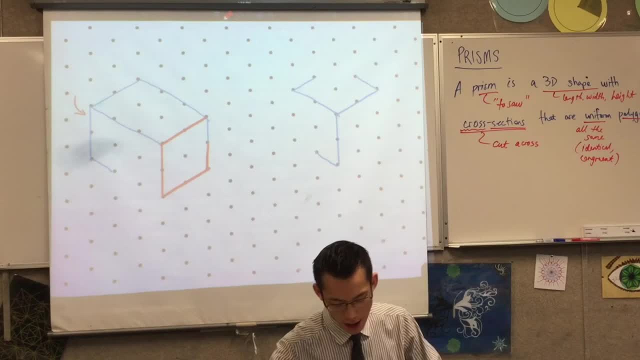 I think we have our complete 3D shape here. I just need to connect the rest of the dots. Okay, so you see it. I just personally. This is just to make things a bit clearer When I draw a shape like this. 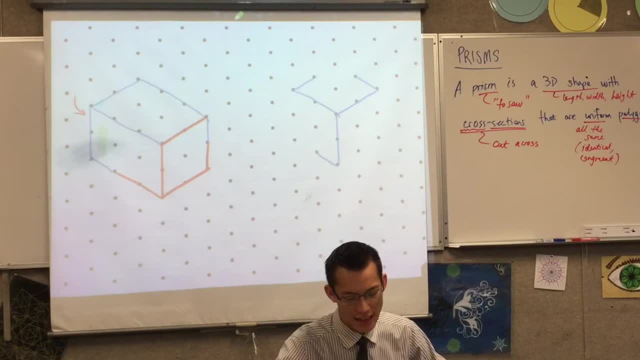 When I draw a shape like this, I think it's kind of nice to add in some kind of shading on one or more. When I draw a shape like this, I think it's kind of nice to add in some kind of shading on one or more. 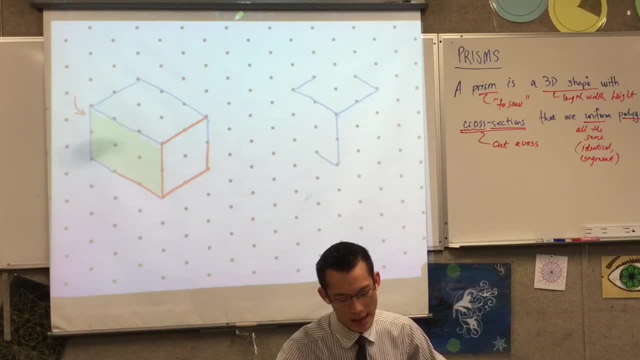 of the faces, because that helps you recognize. hey, this isn't just a flat thing that looks like a hexagon. it actually exists in space and when you look at it from one side, one side will have a shadow, all that kind of thing. all right, let's have a look at this other one. 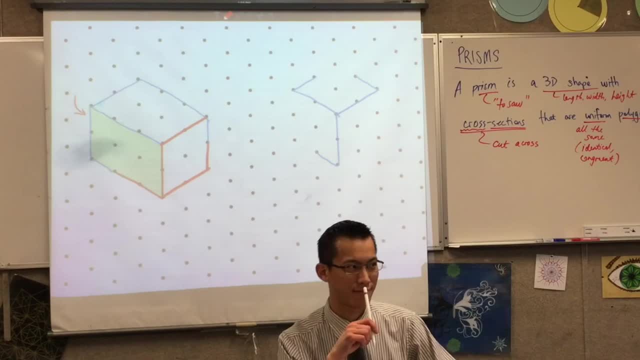 when you look at the other one, you can see again. i'm going to look at all those distances. for instance, can you see this edge here? it goes down two. so therefore, these guys over here, they must go down two as well in order for them to meet. 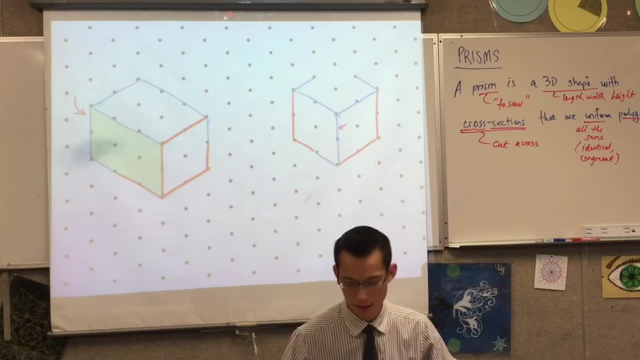 the other edge here, so that's why i'm going to look at the other one. edges that we have parts of. does that make sense? and in the same way from here, you can't just have it coming up here in some random direction. you won't get a prism if you do that right. the only way to 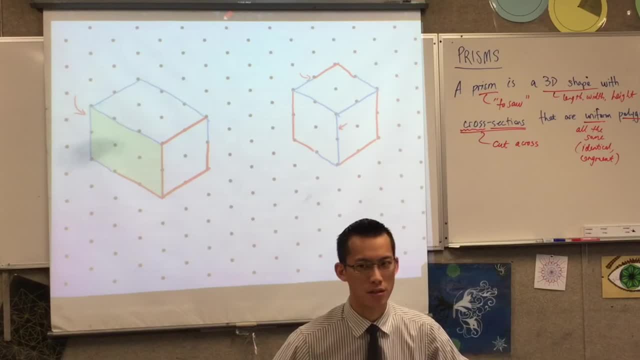 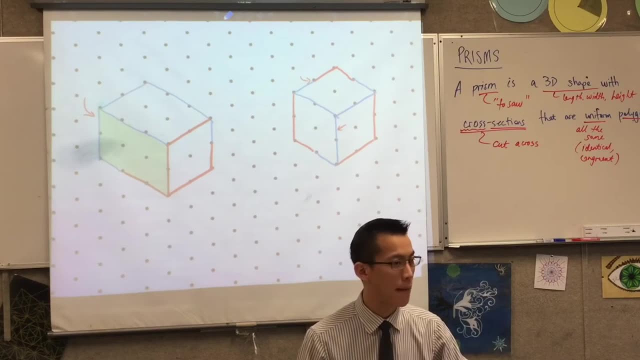 complete the prism is to make sure you've got the same cross section going all the way, okay? so that's the first kind of question. you'll see complete the shape. i will come back to this, so don't worry if you haven't copied it down now. another kind of question is using a 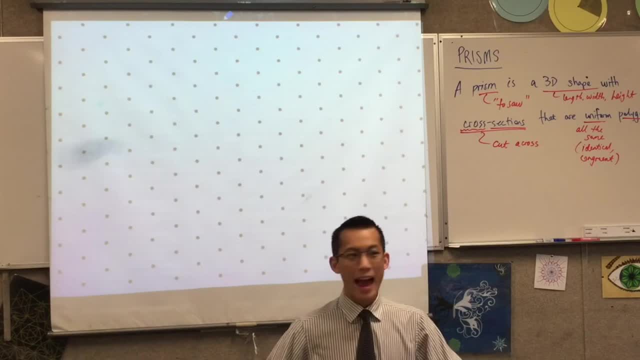 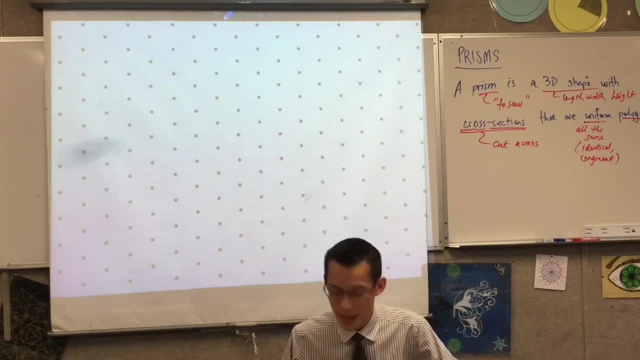 i'm going to guide you and you can draw lots of different triangular prisms to me, but let's do the same one together, just so we get some consistency. for starters, my advice is: start with a cross section. start with one of these polygons that should be the same all the way, ok. so, for instance, i might draw: 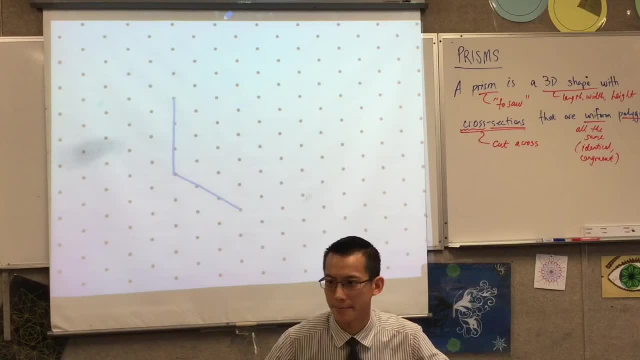 a base and a height like that. ok now, just for the first one. we draw the same class. okay, so i'm going to show you how to draw a bad size Pooruter vor, stone, same one, and then after that I want you to draw a different line. okay now, because this is isometric. 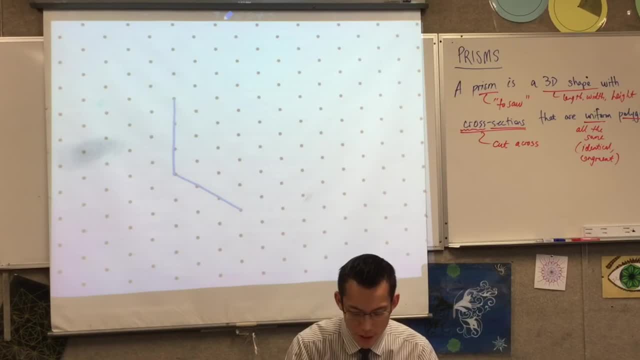 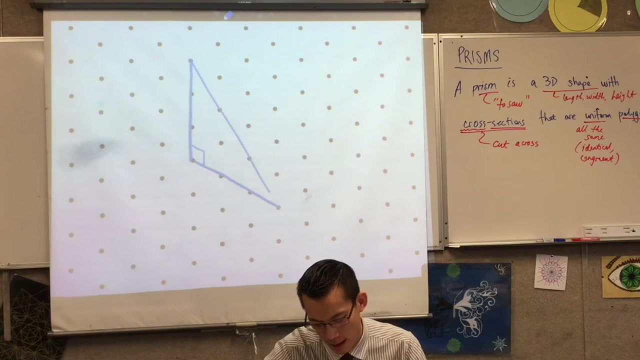 dot paper. we're looking at this object from an angle, so, even though it doesn't look like it- this angle here- I'm doing that as a right angle. okay, can you see, I'm trying to look at that from the edge. okay, I've got two sides here, and now you might like to use your ruler to join these empty. 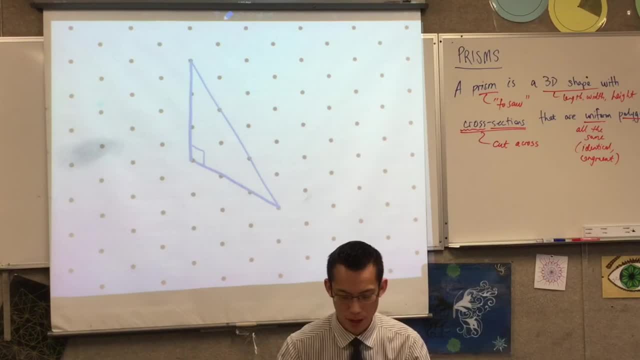 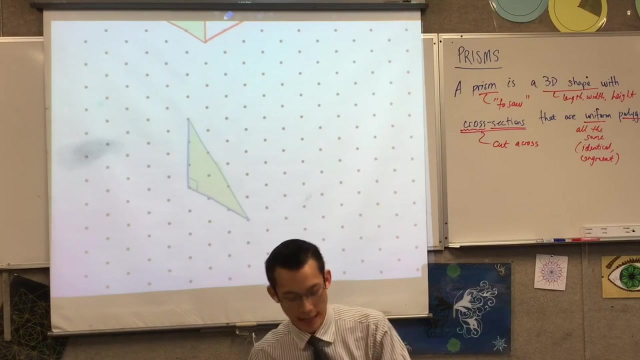 bits up, and if you use the rule, you should get a nice straight edge. okay, so here you go. now, what I've got is this is my cross section in the front right. I should get this same shape over and over again, going off into the distance. okay, so here's what I'm going to do. I'm going to pick a length. 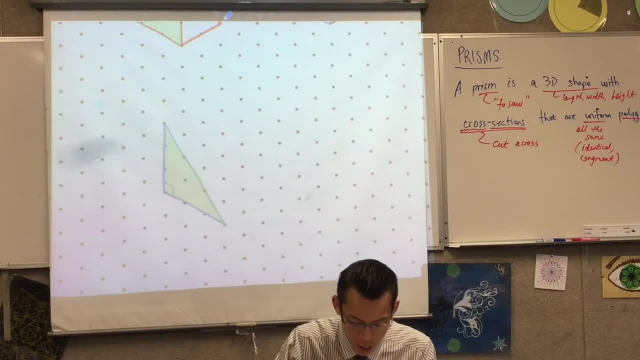 let's make it say: let's go for six. okay, so if I go six units into the distance- one, two, three, four, five, six- I can do that a bit straighter. let's try that again. okay, so that's gone six. you can even for yourself. you can count up because that will help us later on. we're doing 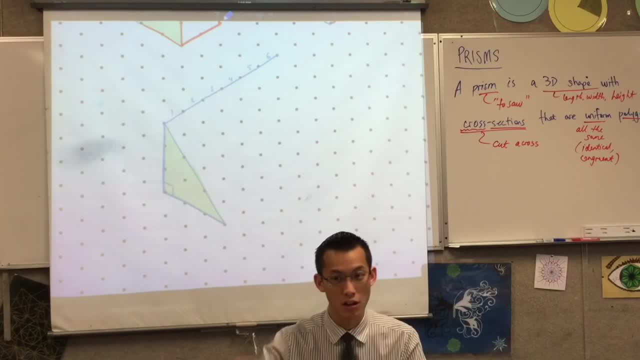 volume. okay, if I've gone six units along the top edge, because I need a uniform cross-section, I'm going to need to go six units along this bottom edge. you see that again: one, two, three, four, five, six. so now to complete this shape, I'm gonna. 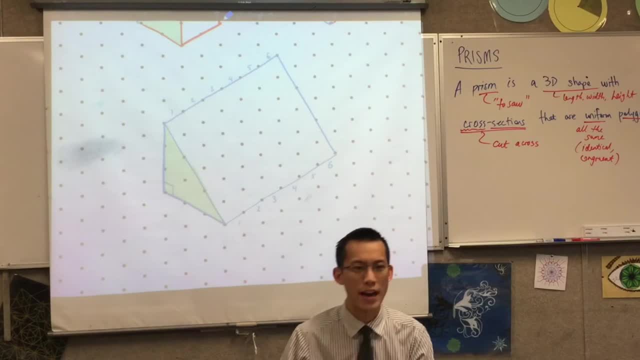 need to join this final edge now, just to finish off this shape. one of the things you often see to make things clearer is that there are edges in this prism that we can't see. there are edges we can't see. so, when you can't see it, when it 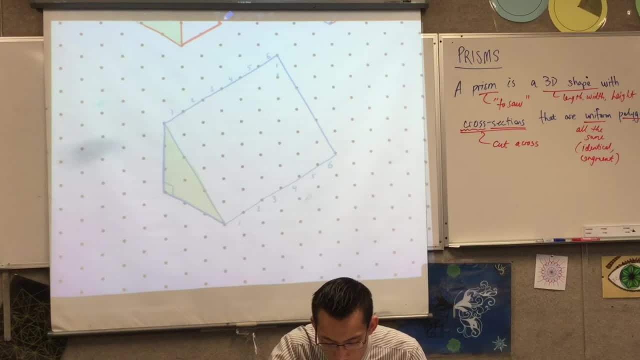 edges are hidden from view. we often draw them in with dotted lines like this: you see those. okay, now quick question for you. how did I know to stop here and not keep on? let me change color and not keep on going like to there. how did I know? yeah, yeah, fantastic. 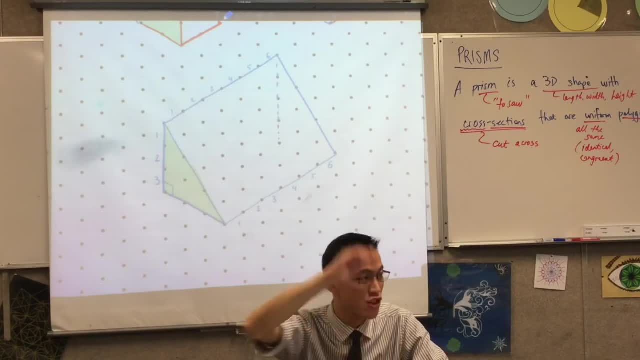 so you see how you can count up and I encourage you write these numbers on there so you can see the count and know how far it's supposed to go. if that vertical edge is one, two, three units long, then this vertical edge over here all the way along into the 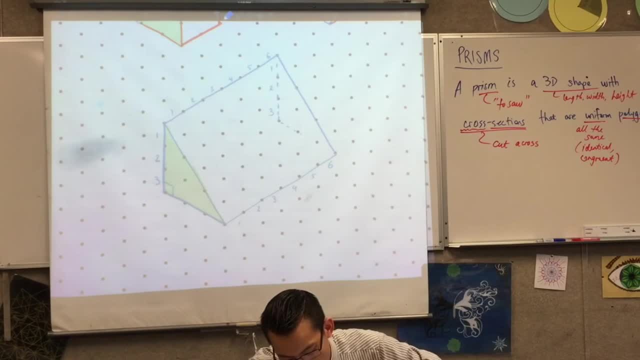 shape should also be three, and then you can complete it over here. there's one edge missing. how long should it be? look carefully how long it should be: six right, six all the way along here and now. if you've drawn it like I have, you can actually see: yeah, that looks pretty 3d, even though you've actually done it. 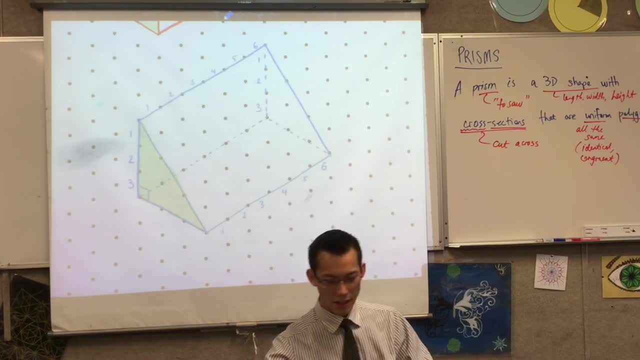 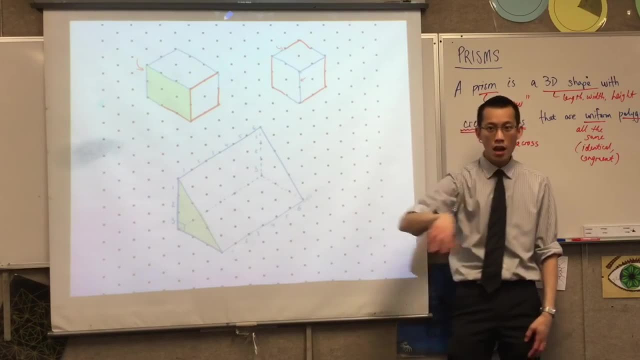 right on a 2d piece of paper. I know nice, okay. so what I'd like you to do now is I just, um, I just guided you through these three shapes. right now, while you've got in front of you, can you draw another triangular prism for me? but draw 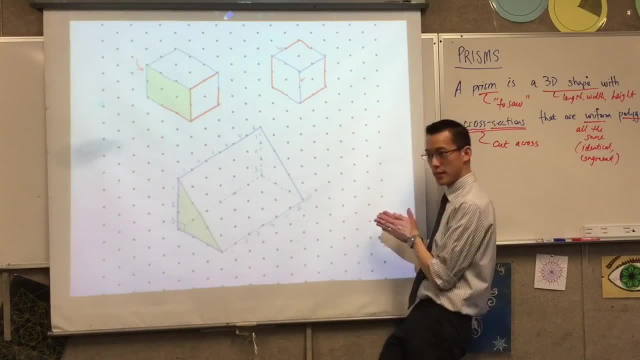 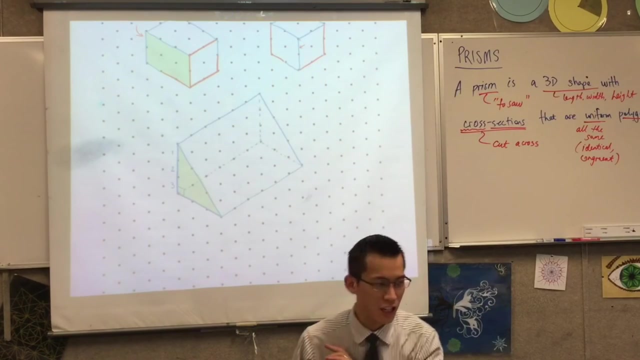 it differently. maybe you don't want to facing this way, maybe you want facing that way or facing down. maybe you want the triangle on the top. draw a different size triangle, anything you like. once you've got one, call me ever. I'd like to have a look at it and I'll see if we can pick up some of the best. can I just show? 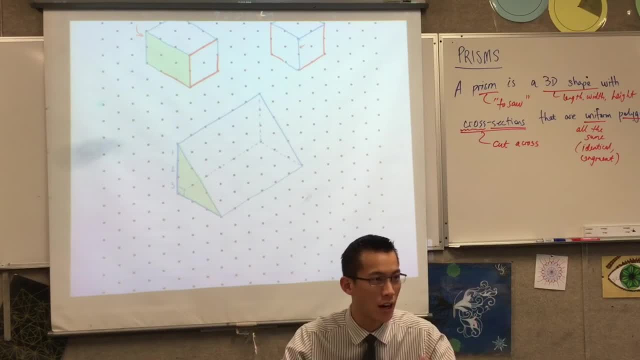 you one last thing, because I want you to finish off all those prisms at home, make some new ones, whatever you want to do, and I'll see you in the next video. bye, bye, beautiful, well done. can you just look up for a minute, because I've seen some?